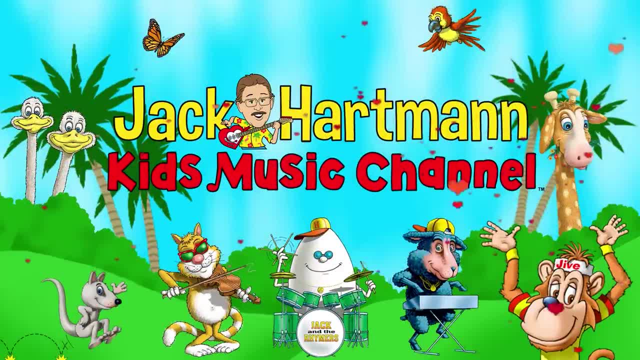 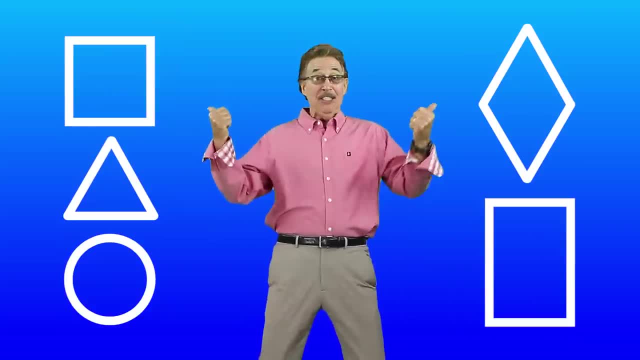 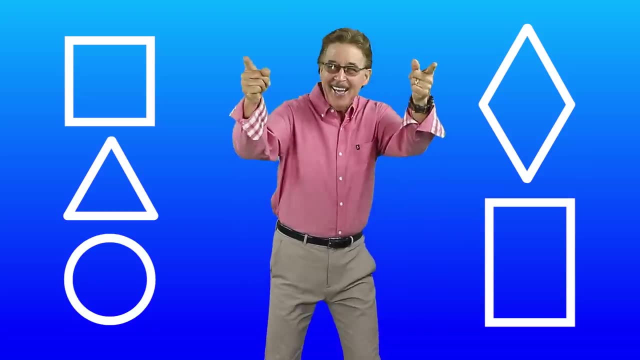 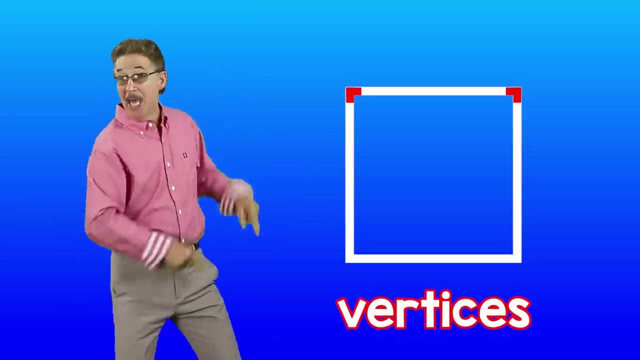 Jack Cartman Kids in the Channel 2D shapes: 2D shapes: Which ones have sides and vertices? Let's learn today. Sides are the straight lines that form the shape. Vertices are the corners that the two lines make. Let's move and count the sides and vertices of these 2D shapes. 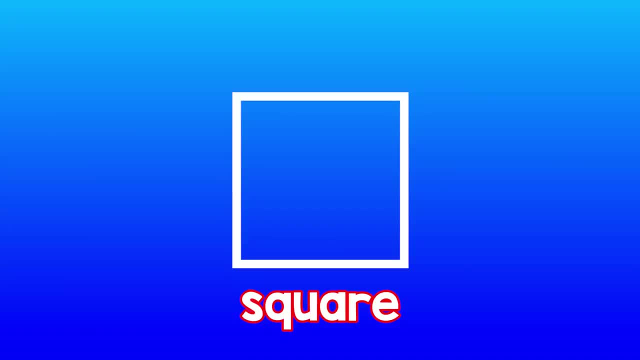 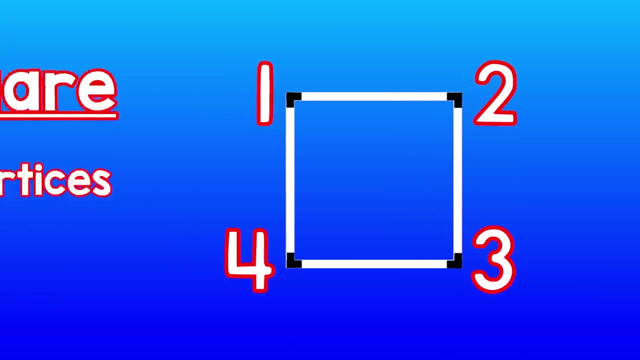 This is a square. Let's move and count the sides of a square: One, two, three, four. A square has four sides. Let's move and count the vertices of a square: One, two, three, four. A square has four vertices And four sides. 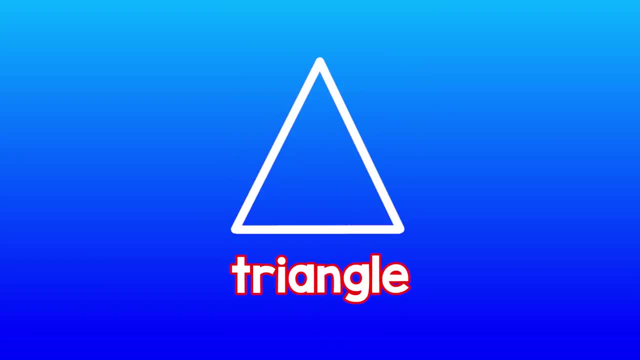 This is a triangle. Let's move and count the sides of a triangle: One, two, three. A triangle has three sides. Let's move and count the vertices of a triangle: One, two, three. A triangle has three vertices And three sides. This is a rectangle. 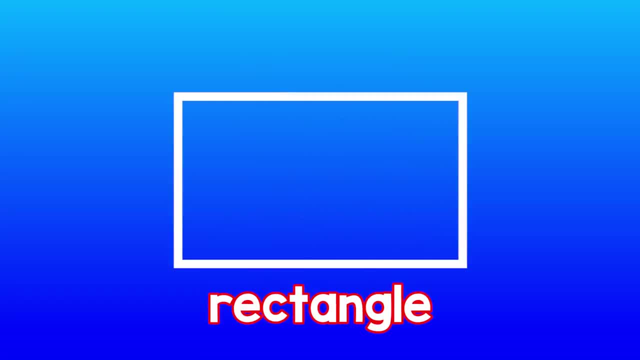 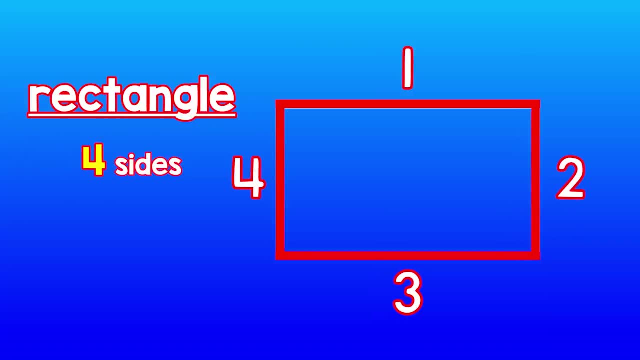 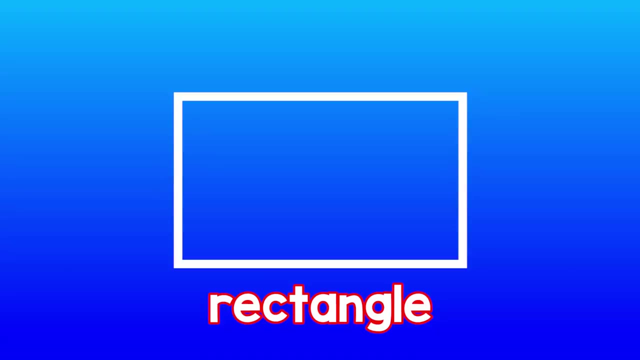 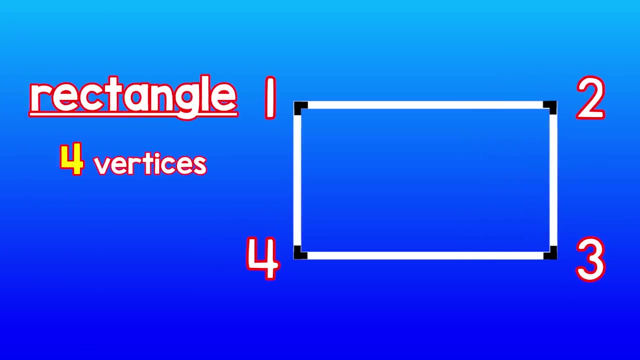 Let's move and count the sides of a rectangle: One, two, three, four. A rectangle has four sides. Let's move and count the vertices of a rectangle: One, two, three, four. One, two, three, four. A rectangle has four vertices and four sides. 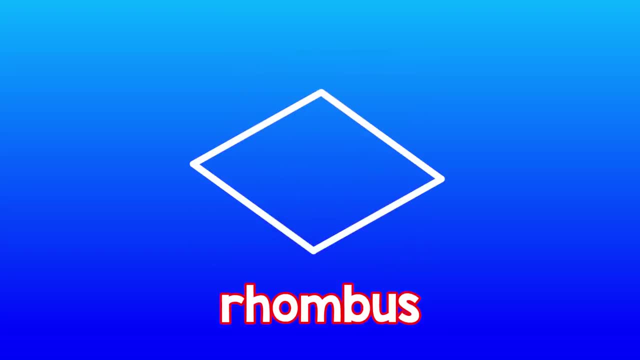 This is a rhombus. Let's move and count the sides of a rhombus: One, two, three, four. A rhombus has four sides. Let's move and count the vertices of a rhombus: One, two, three, four.